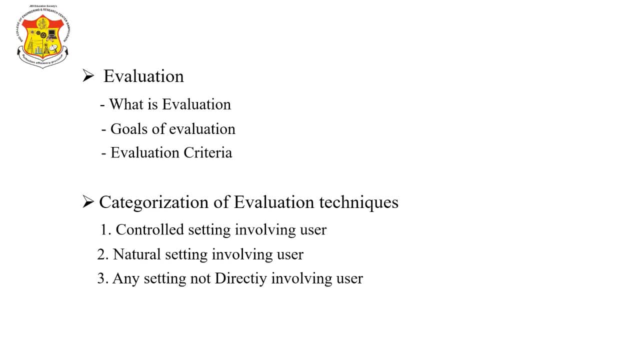 this evaluation it is, you can say. it is needed to access the desires, the designs and test system to ensure that they actually behave as a user aspects and meet user requirements. This is the rule of this is the rule of evaluation. Evaluation should not be thought of as a single. 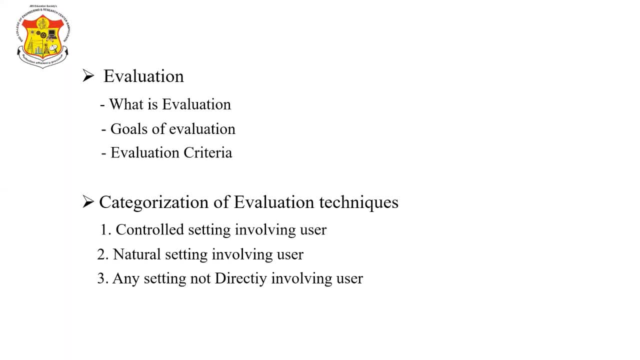 phase in design process. Evaluation should occur throughout the design life cycle, with the result of the evaluation feeding back into the modification to the design. So what are the different goals of design, or goals of evaluations? So the first goal is there. I mean there are mainly three. 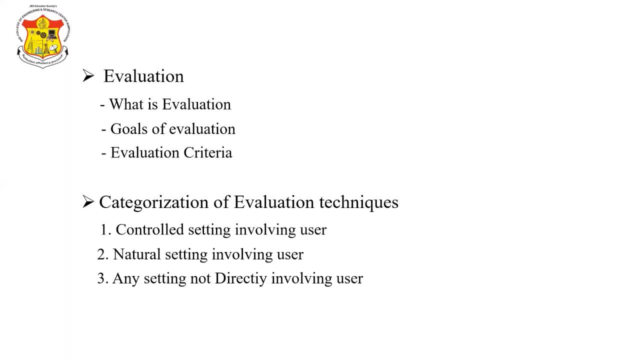 main goals for this evaluation. First, To assess the extent and accessibility of the system functionality. So what do you mean by this? So this includes not only making the correct functionality available within the system, but making it clearly reachable by the users in terms of 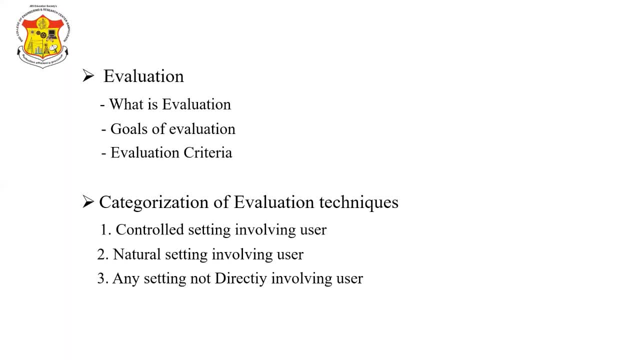 action that the user needs to take to the carry out the task. It also includes matching The use of system to the user's expectation of them does. second, to assess the user experience of the interaction. So this second goal includes the considering features such as how easy the system is to. 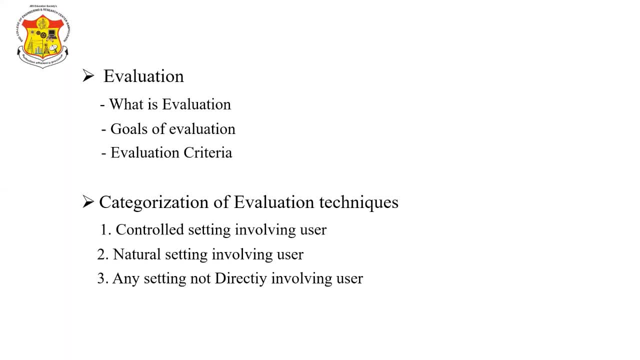 be understand its usability and user satisfaction with it does. it may also include his enjoyment, and emotional. So the third goal is to identify the problem that the user needs to solve and use in response, particularly in case of systems that are aimed at a- you can say that an- aim at the entertainment. 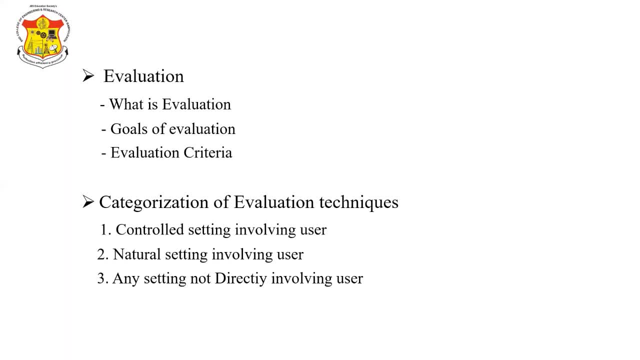 Third one, to add NT, you can say, to identify any specific problems with the, with the system. This, this is the third goal. So in this goal, this, this is a correlate To the, both the functionality and usability of the design. 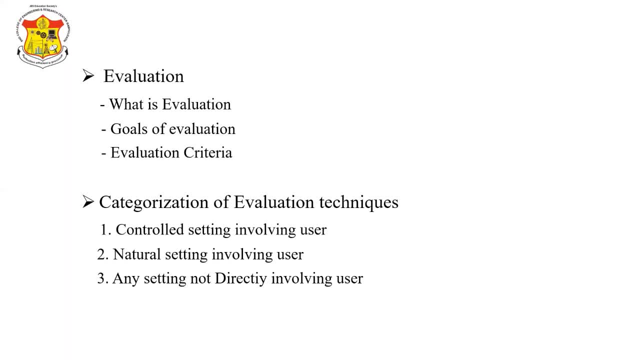 It is specifically concerned with the user. So this is the third goal. So the fourth goal with the identifying trouble spots which can be rectified. so these are the three different goals of evaluation. so what is the evaluation criteria? so fuller classification of usability principles, including learnability, flexibility and robustness, can be used as evaluation criteria. 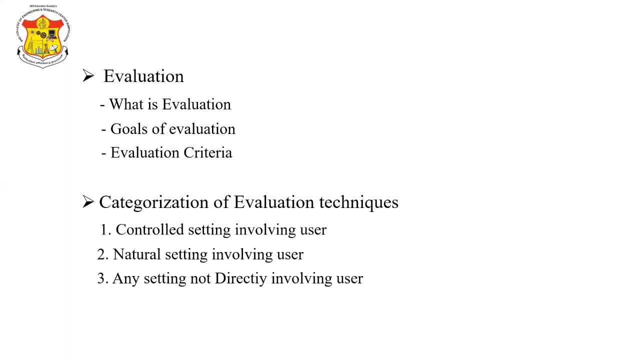 so this evaluation is aimed at measuring this features. so we will see latter. what are the different classification of this evaluation? so next, there is categorization of evaluation techniques. so, depending on the setting- user, participation and control level- evaluation is classified into three large categories. first, there is control setting involving users. second, a natural setting involving users. and. 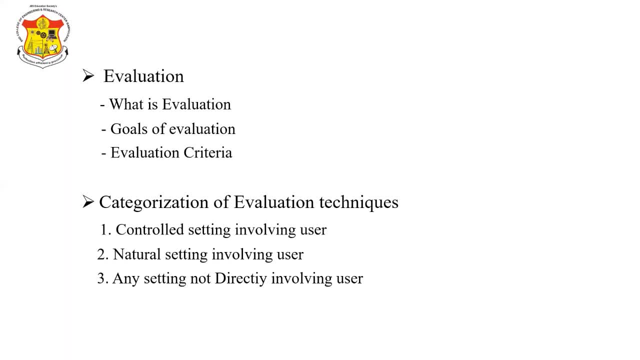 third one is any setting not directly involving users. so this control, user setting, the activity of the user is controlled by the hypothesis and measurements or compliance, the usability test and experience are the main methods. natural user setting that is, we can say the user activities can be determined little. 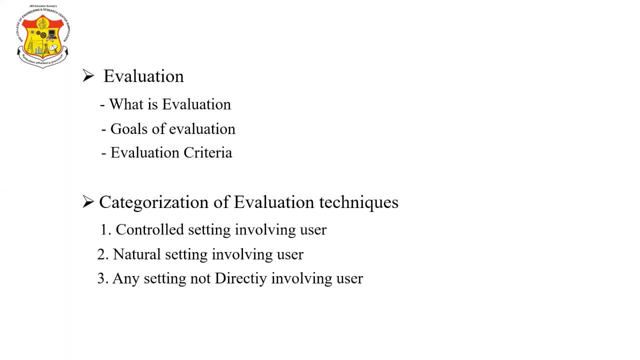 or no control how the real world that product would be used. field studies are main method used in this natural setting involving user. then there is any setting that do not include user directly. the most obvious usability problems are criticized by consult consultants and investigators for predicted and model aspects of the 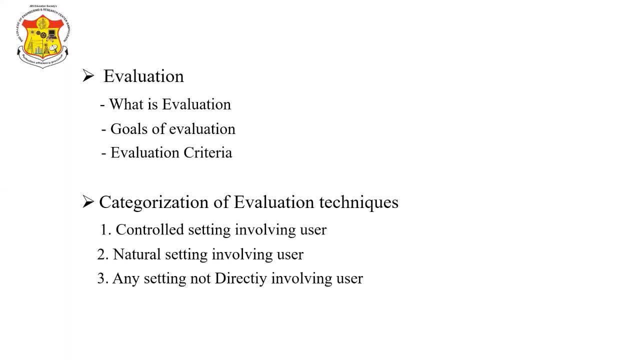 interface. the methods cover inspection, heuristics, pathways, models and analysis, so we'll see this three categories in detail. so in control setting involving users, the experiments and user tests are designed to control what user do, when they do it and how long they are designed to reduce. 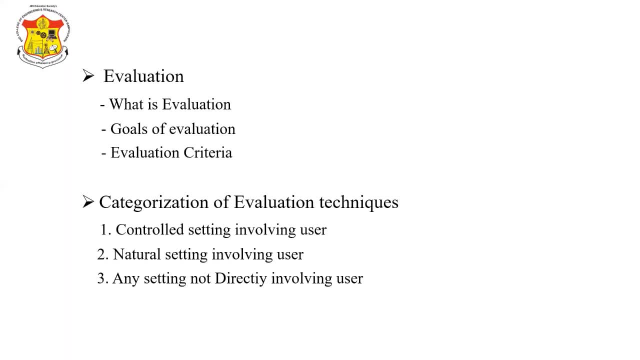 outside influence and distractions that might affect the results, such as people talking in the background, experiments and user tests. tests are designed to check what users are doing, how long they are doing it. they are intended to use external influence and distraction for example, For example, those who speak in the background. the approach was extensive, used successfully. 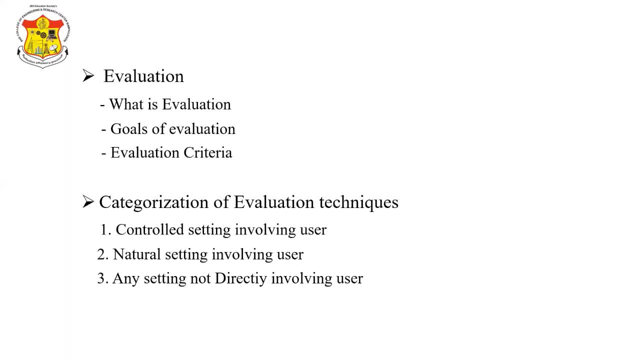 to elevate the laptop and other device software applications where the number of tasks can be performed by the participants. Second, there is natural setting involving users. examples you can see are publicly available online communities and products. The activities of the users are little or no control to determine how the product is. 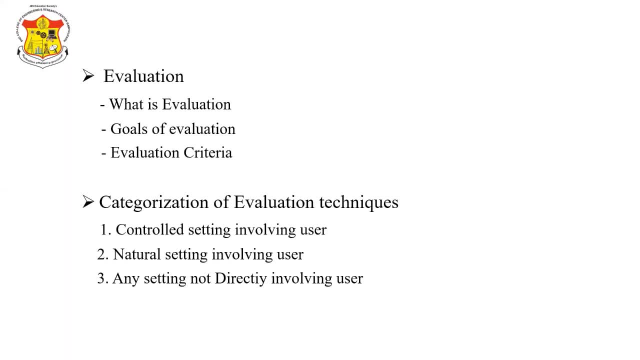 used in the real world. Field studies are principal way. The aim of field studies is to access the product in their natural environments with user. The main purpose of field studies is that is first, help identify opportunities for the new technology. Next they establish the requirements for the new design and third, that is, facilitate. 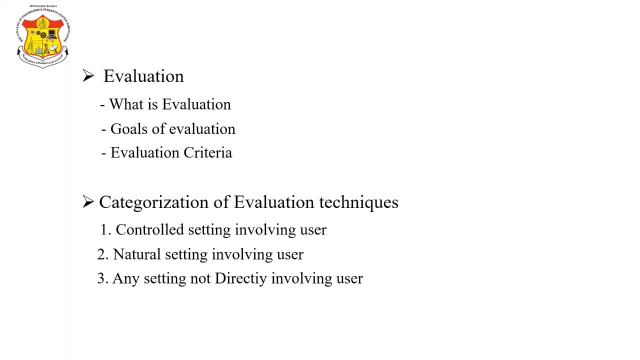 the introduction of technologies or inform deployment of existing technology. in the new context, The data recorded by the researchers as a note or the notes, or via audio or video recording, or by those participants as a journals and notes. The data is used as an event and conversations. 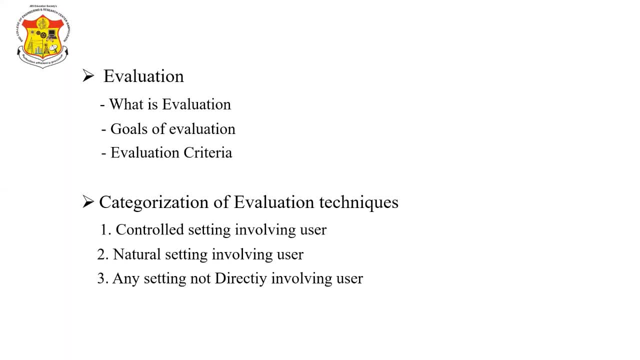 The goal is to be discreet and not be influenced. what people do evaluation. During the last 15 years there has been a trend towards conducting in the world- you can say in the wild- studies. These are essential user studies that look at how new technologies or prototypes that 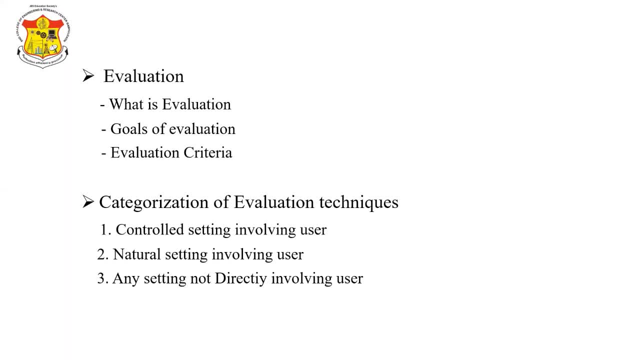 have been deployed, Any used by people in various settings, such as you can say there is outdoors, in public places and in homes. The downside of handing over control is that it makes it difficult to anticipate what is going to happen and to be present when something in the state does happen.